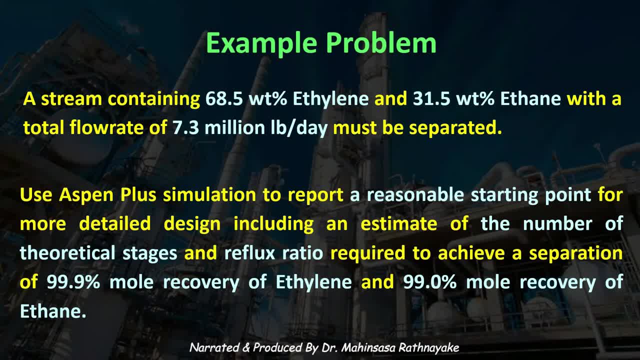 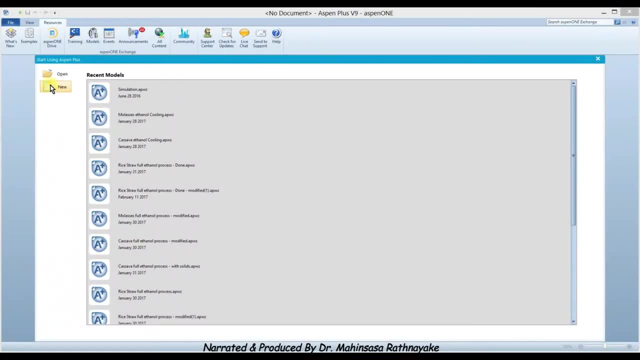 We have to estimate the number of theoretical stages and reflux ratio required to achieve a separation of 99.9% mole recovery of ethylene and 99% mole count. percent mole recovery of ethane. Open a new Aspen Plus simulation by selecting new blank simulation and click create. 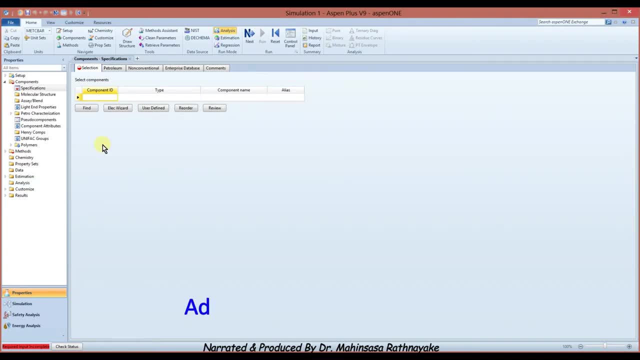 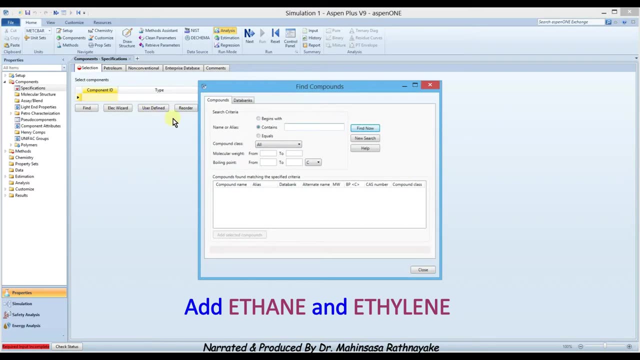 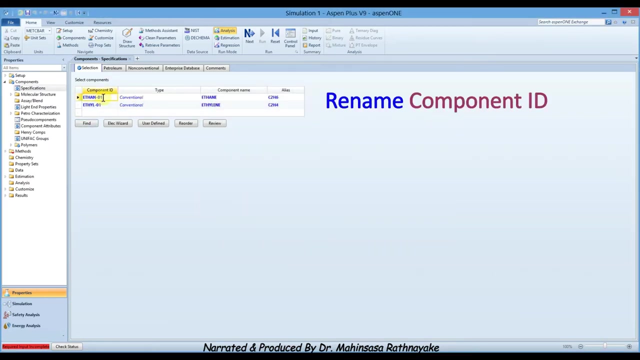 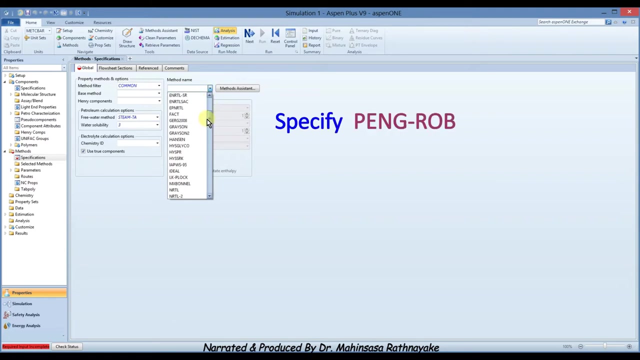 In the components tab, enter the components needed for this simulation. So we enter ethane and ethylene And that's it Then click next. We have to define the valid property method. Select Penrobinson as the base method. The Penrobinson equation of state is typically: 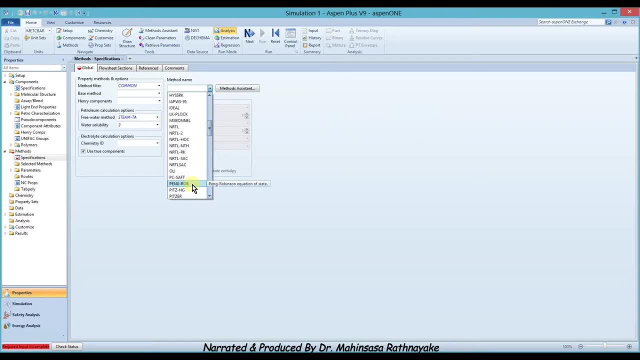 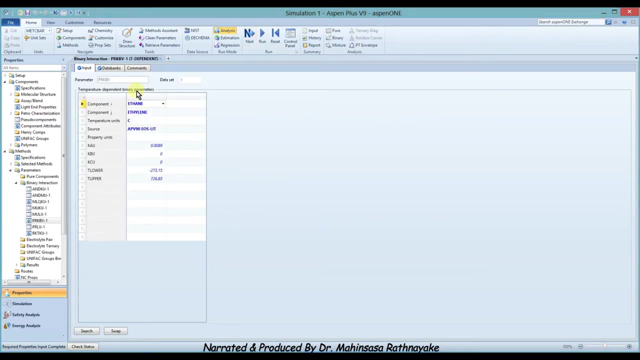 used to model systems containing hydrocarbons at high pressures. Since our system has only ethane and ethylene, this is the most valid property method. Populate the binary interaction parameters by clicking next button. Then click the next button again and run the property analysis. Then go to the simulation environment by clicking the. 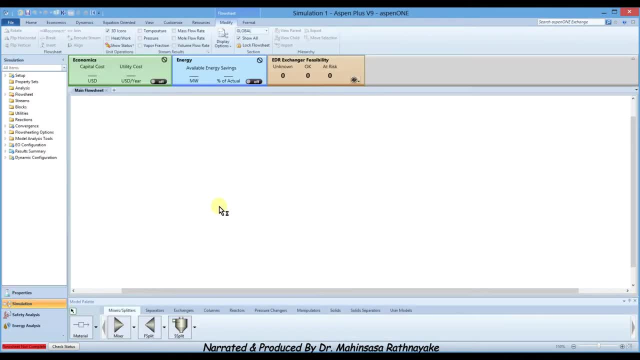 simulation button below. From the models library go to columns section and insert a DSTW view block into the flowsheet. Then connect the feed stream to the column input and distillate stream at the top and the bottom stream at the bottom. Rename the stream and the distillation column block with proper names. 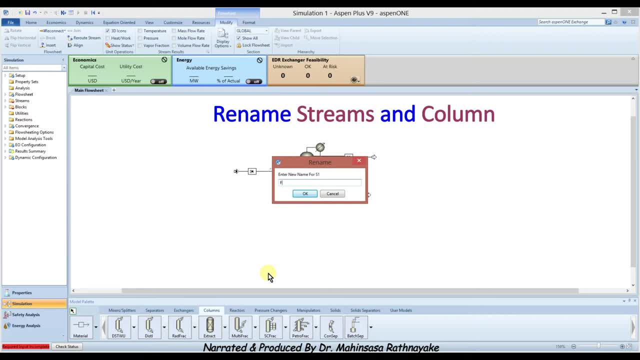 Now create a new flow sheet with the same names and a field of EU4 At the top. the field of EU4 will be shown as the field of EU2. If you don't have an enough field of EU2, you can use the field of EU2. 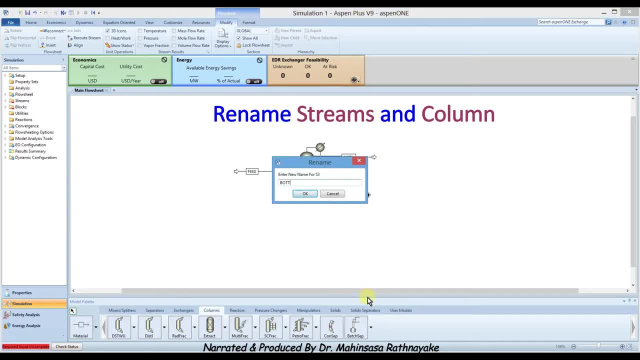 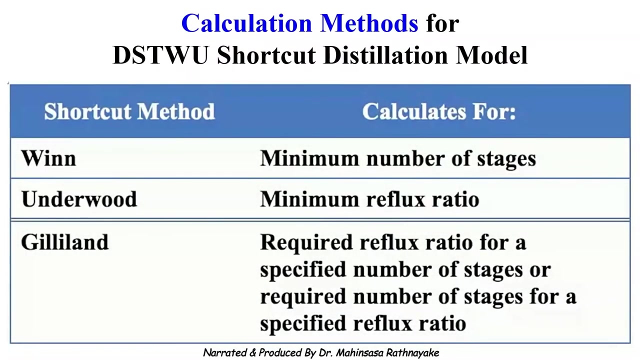 in the distribution box. The field of EU2 can be defined as a field of EU3. We'll discuss that when we're done with this video. The DSTW block uses the semi-empirical equations to estimate the separation. The Winn equation is used to estimate the minimum number of theoretical stages. 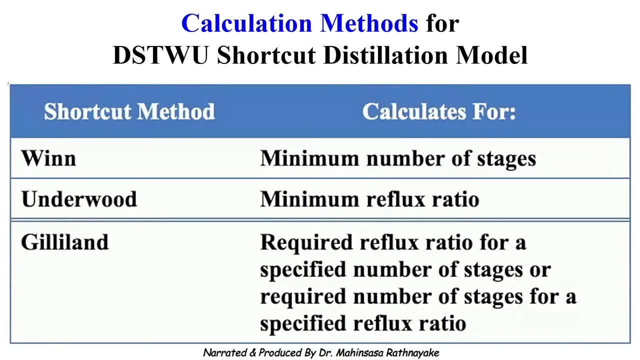 The Underwood equation is used to calculate the minimum reflux ratio. The Gilliland equation is used to calculate the required reflux ratio at a specific number of stages or the number of stages at a specified reflux ratio. If you want to know more details about this block, go to AspenPlus Help and type DSTW in the index. 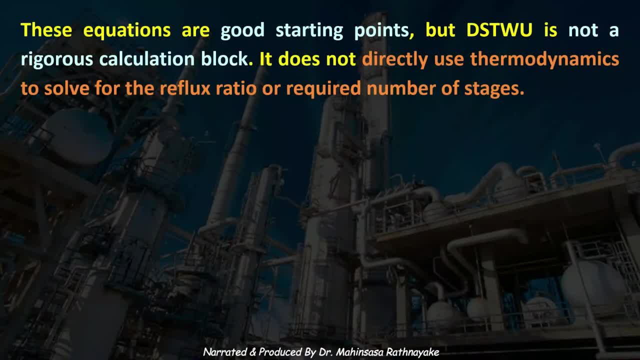 These equations are good starting points, but DSTW is not a rigorous calculation block. It does not directly use thermodynamics to solve the reflux ratio or required number of stages. Therefore, rigorous, look at this separation block. The DSTW problem should be redone using the Red Fract Distillation Column model. 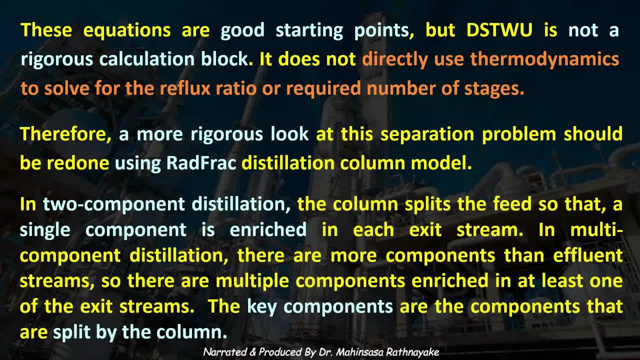 In two-component distillation, the column splits the feed so that a single component is enriched in each exit stream. In multi-component distillation, there can be more components in each stream. The key components are the components that are split by the column. 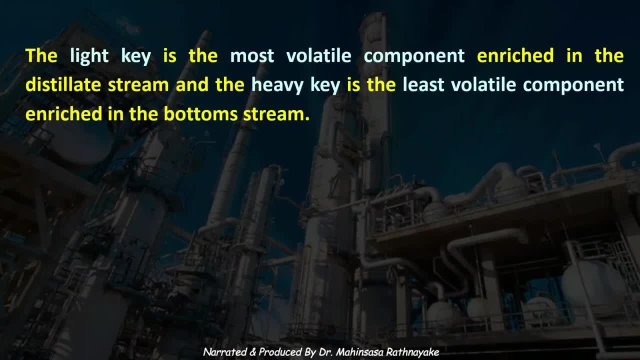 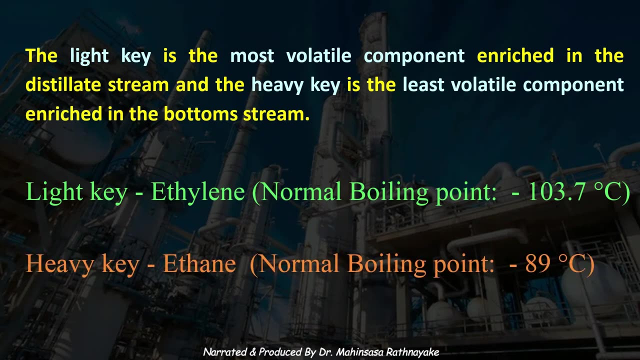 The light key is the most volatile component which is enriched in the distillate stream. The heavy key is the least volatile component enriched in the bottom stream. So in our problem, the heavy key is ethane and the light key is ethylene, because the ethylene has a lower boiling point than ethane. 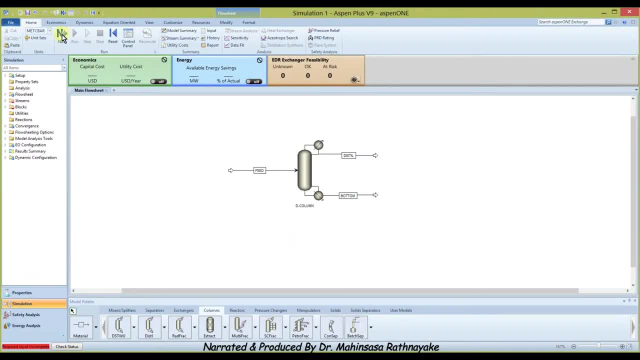 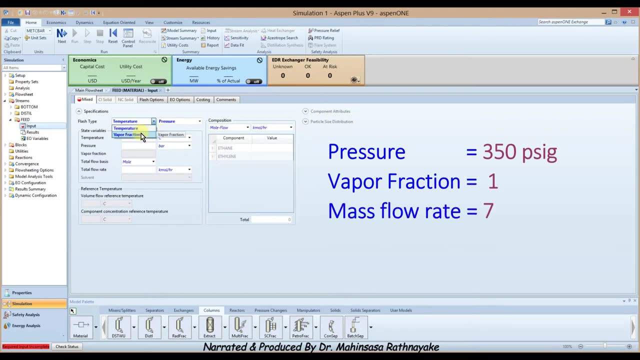 After the flow sheet is complete, click next. Enter the feed stream data. Select the flash type variables to be pressure and vapour fraction, because we need to estimate the temperatures in each stream. Enter the pressure as 350 psig and vapour fraction as 1.. 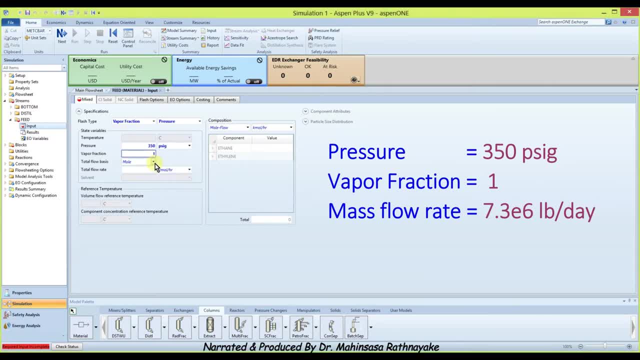 Enter the total flow basis oz per day and enter the value as 7.3 million. Enter the composition of the feed stream as mass fraction of 1.. Enter the ethane: 0.315 and mass fraction of ethylene: 0.685.. 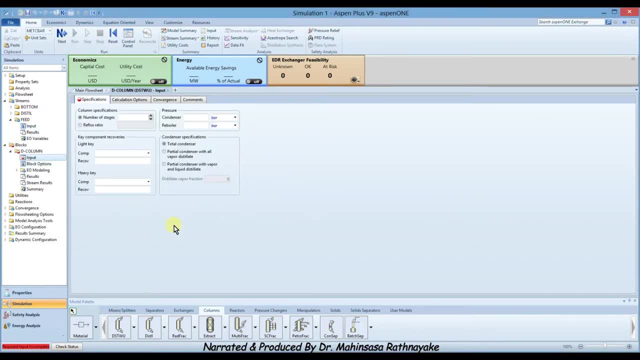 Click next. Go to the column block setup. In the column block setup, enter the number of stages as 30.. Select the light key as ethylene and heavy key as ethane. Enter the desired recoveries for these components in the distillate stream. 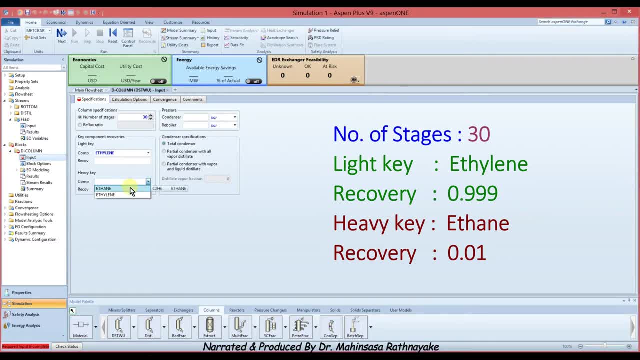 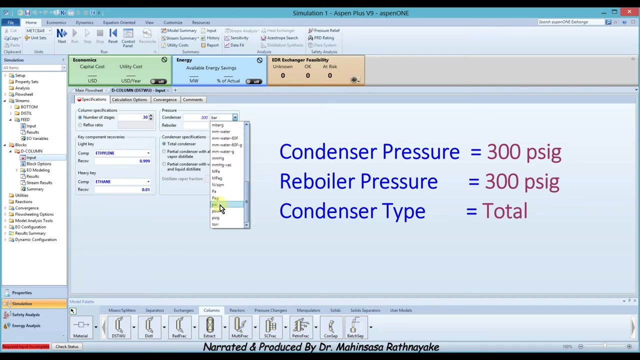 So that 99.9% ethylene recovery in the distillate stream and 1% recovery of ethane in the distillate stream. Then enter the condenser and reboiler pressure to be same as 300 psig. Select the condenser specifications as total condenser. 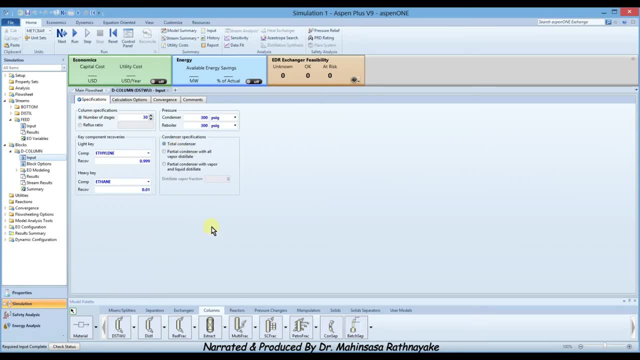 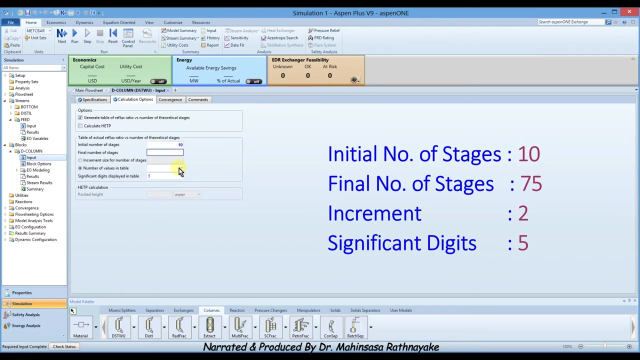 Then go to calculation options and select the generate table of reflux ratio versus number of theoretical stages option. Enter reasonable estimates for the initial and final number of stages. So we enter initial number of stages as 10 and final number of stages as 75.. 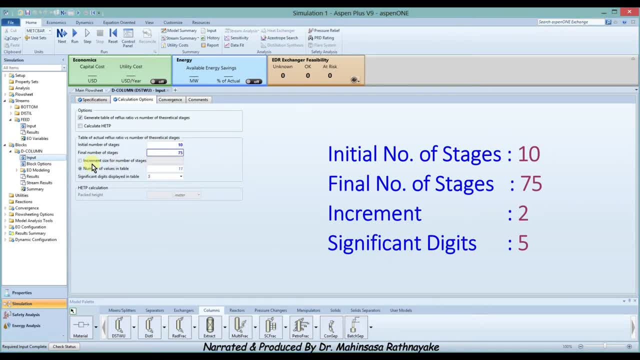 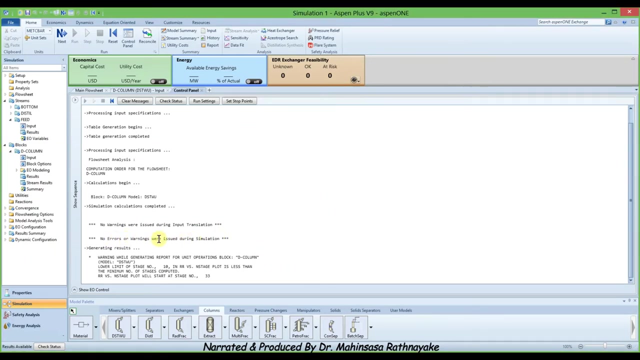 Then enter an increment size as 2.. Also select the significant digits displayed in table as 5.. We have entered all the input data for this initial simulation. Click next and run the simulation. The simulation runs without any errors. To see the results: table for reflux ratio versus number of stages. 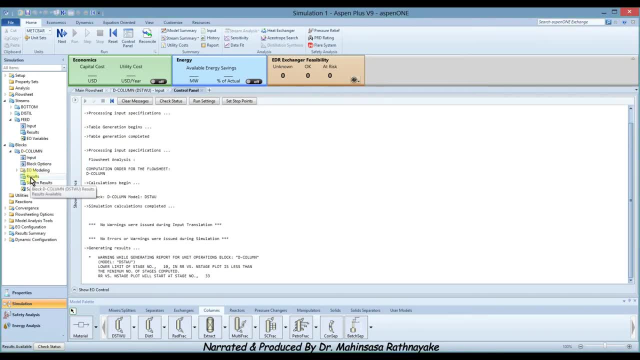 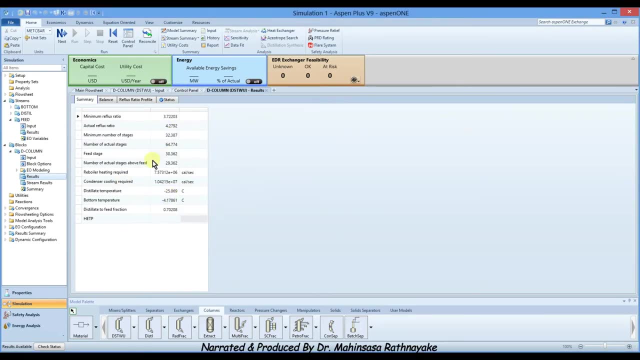 Go to reflux ratio: profile tab of the results page for the column. The column results page is available in the navigation pane So we can see that a results table is available with theoretical stages and reflux ratio. We can copy and paste these values into Microsoft Excel software. 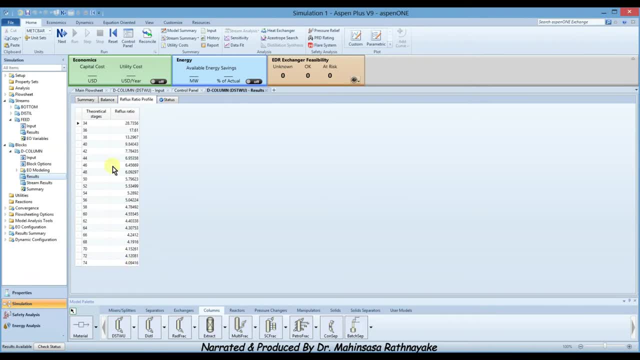 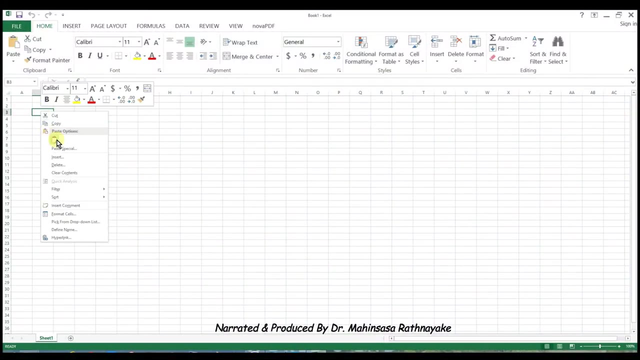 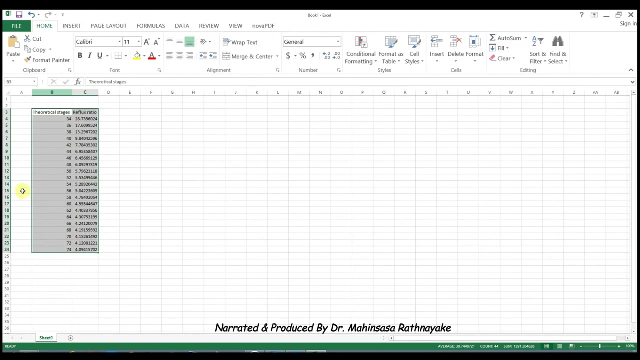 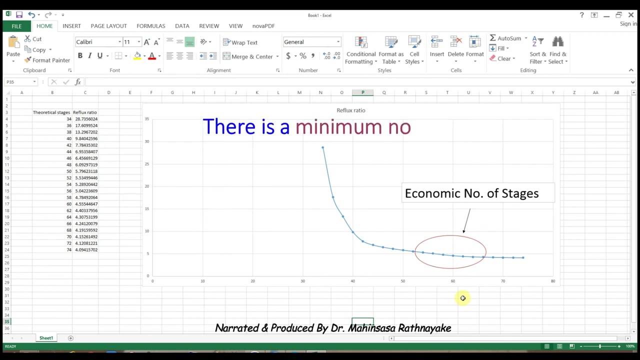 So copy and paste into Microsoft Excel software and we can generate a graph using these values. When we have a look at this graph, there is a minimum number of stages for a given separation. And when we have a look at this graph, there is a minimum number of stages for a given separation. 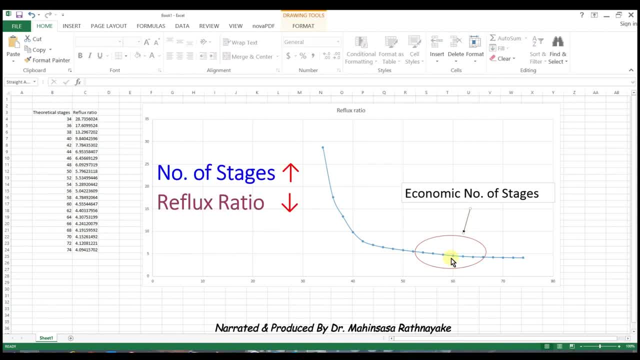 And when the number of stages are increasing, the reflux ratio is reducing and becomes stable. Increase in the number of stages will increase the capital cost of the column. Increase in the reflux ratio will increase the operating cost of the column Because more material is recycled and it must be reheated in the reboiler and recondensed in the condenser. 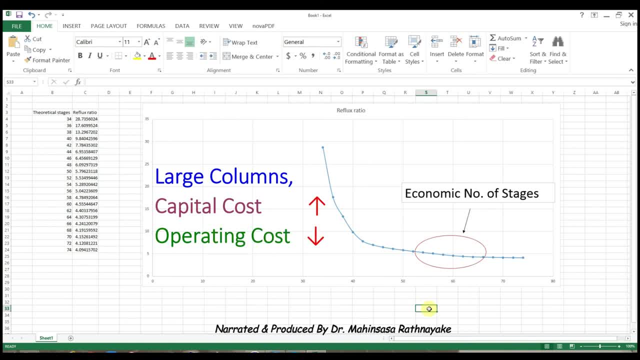 Therefore, larger columns have a larger upfront cost but lower operating cost, While smaller columns have smaller capital cost but they are more expensive to operate. So we have to select an economic optimum between these two trade-offs using this curve. So according to these simulation results, we can suggest that around 60 number of stages is more suitable. 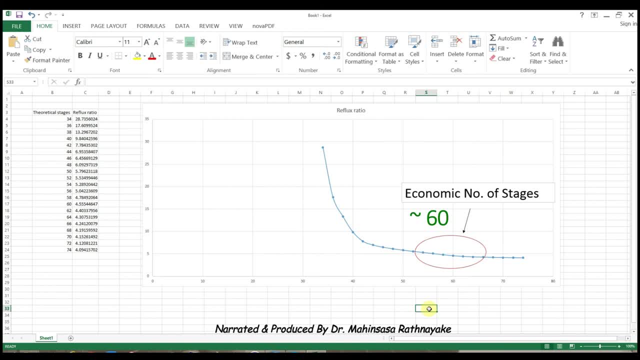 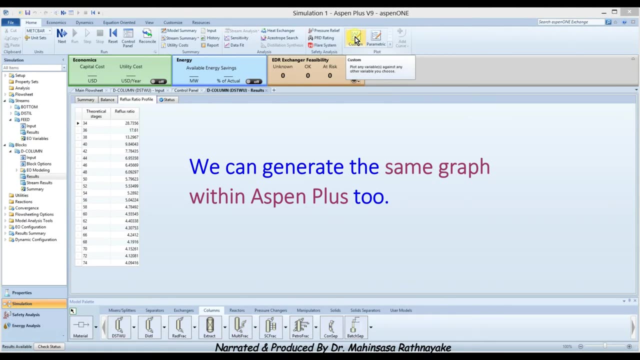 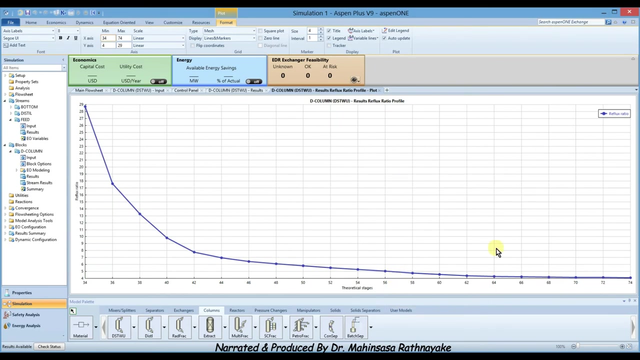 considering both operating cost and capital cost. However, a real distillation column will need slightly more stages to achieve the separation model in this DSTW block. However, a real distillation column will need slightly more stages to achieve the separation model in this DSTW block.